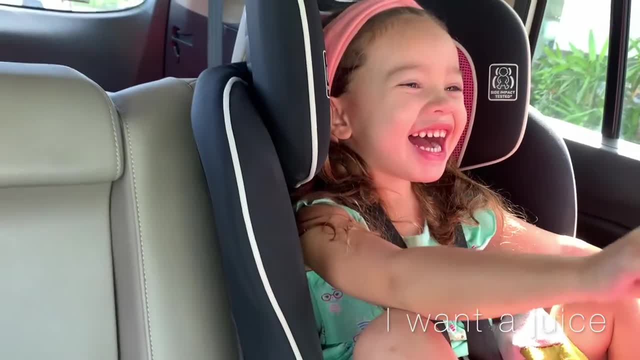 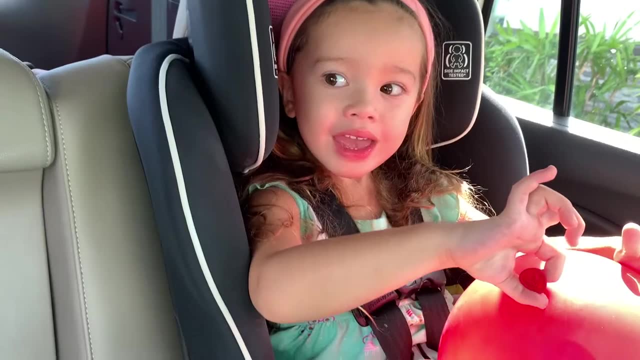 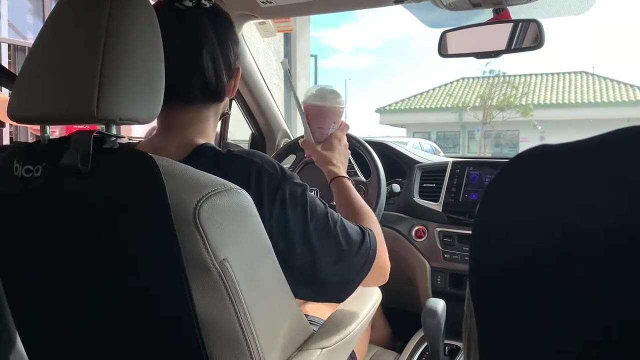 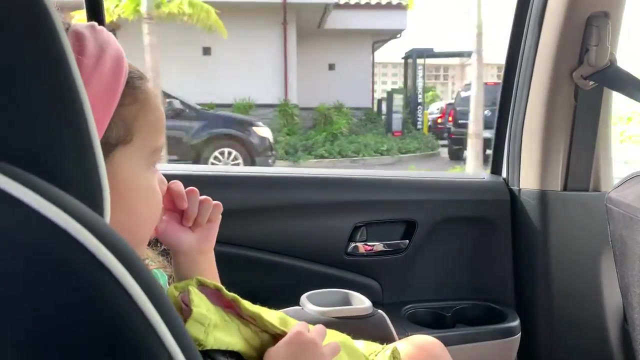 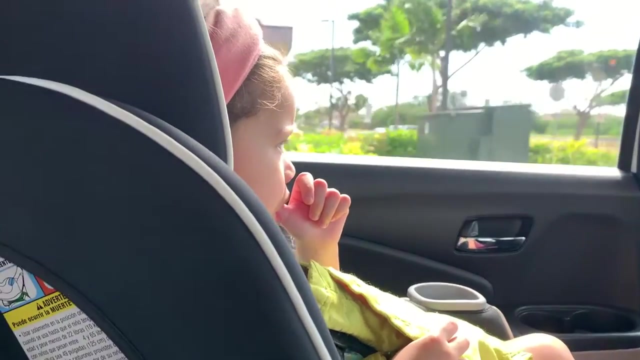 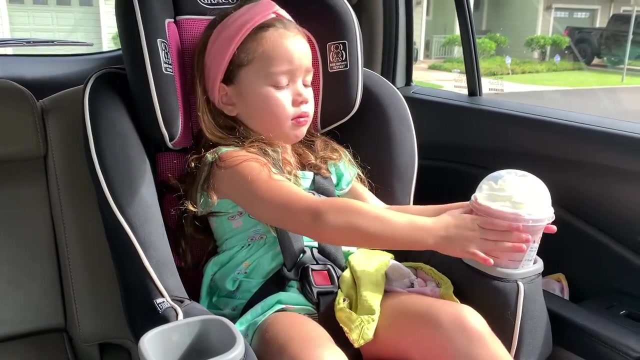 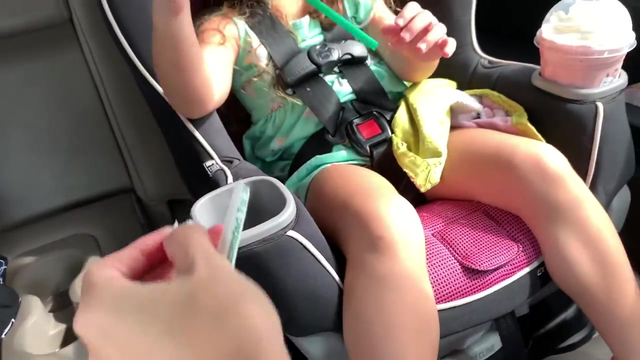 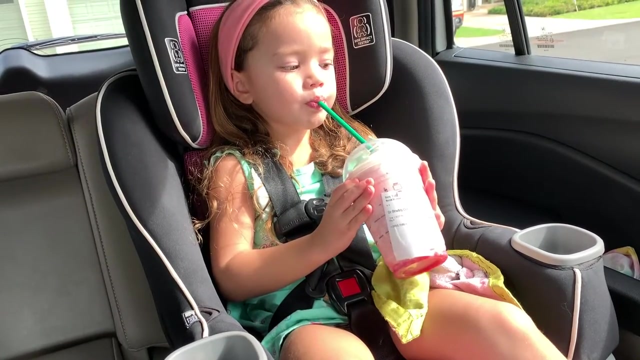 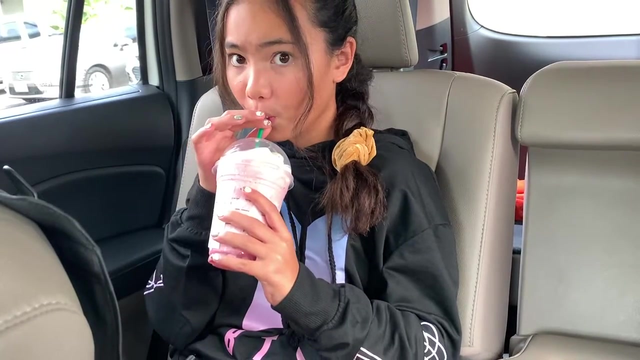 caffeine, um, and this is also strawberry too. it's like strawberry, so, and you put it with sugar and it tastes like strawberry. where's the straw? give the babies this straw give. i can open it on myself. how is it good? you get in trouble. that's good. 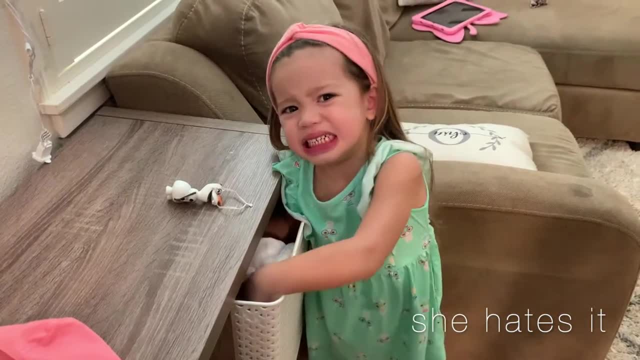 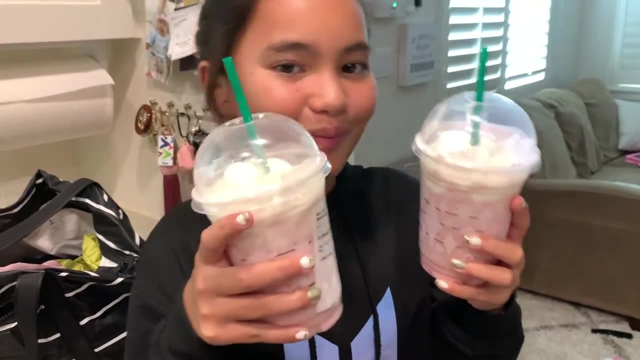 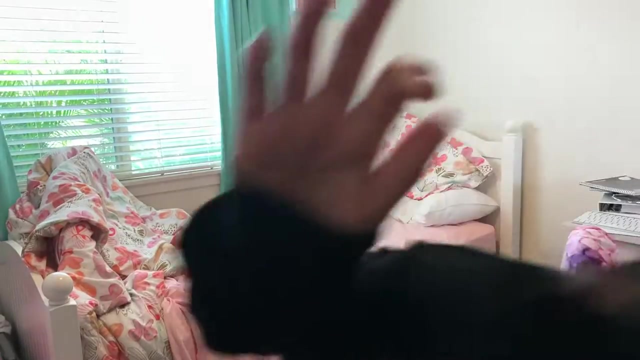 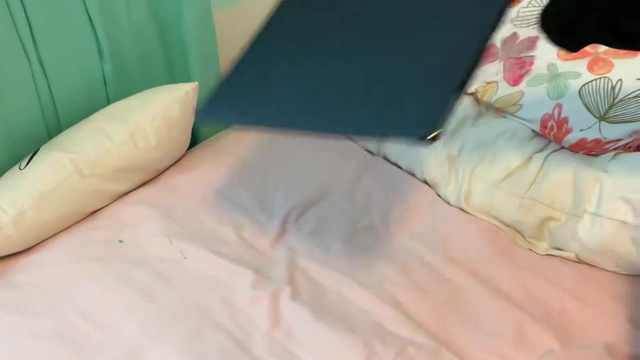 i guess i get to have both, all right, so we got our starbucks and now we're ready to start cleaning. okay, so the first thing we're gonna do is clean up my bed, so let's get started. it's 1, 12 a 5 in the house. 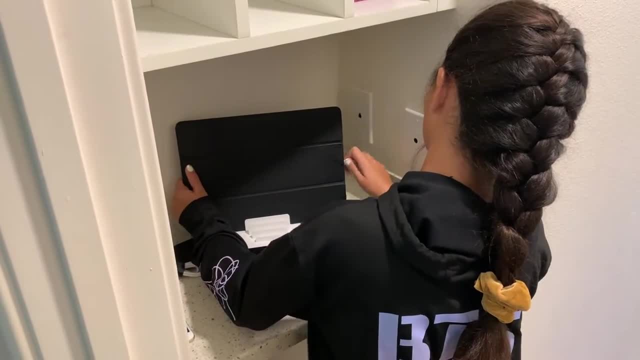 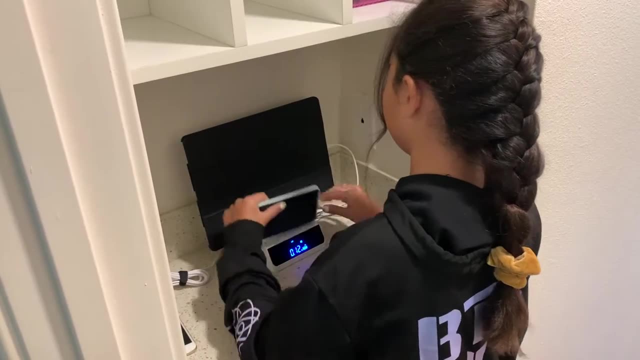 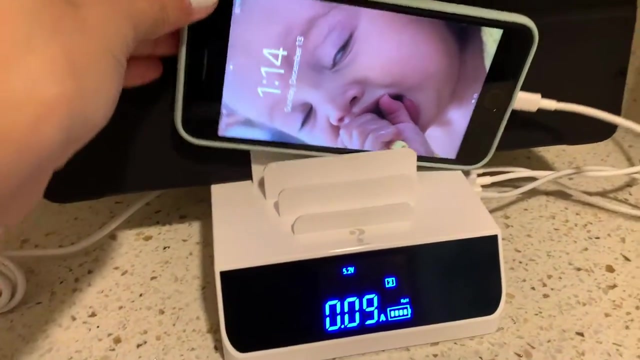 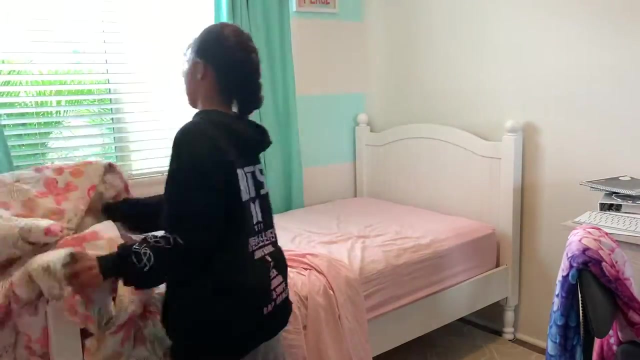 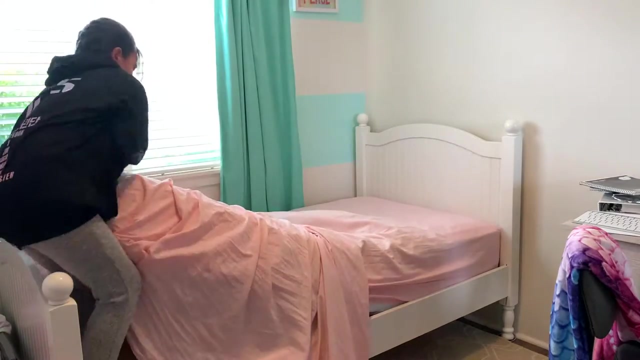 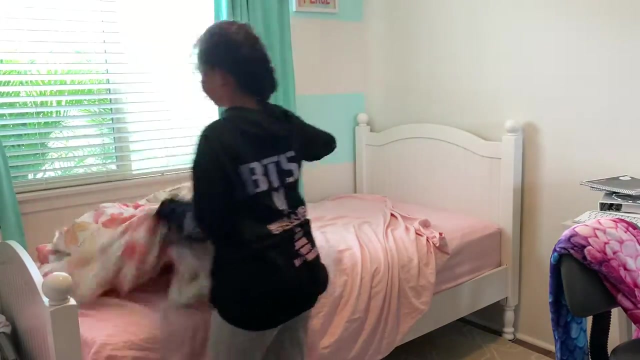 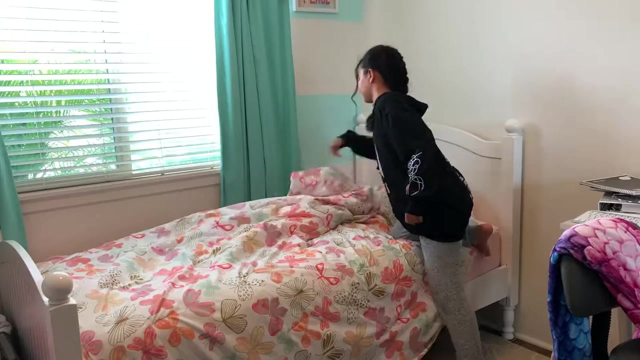 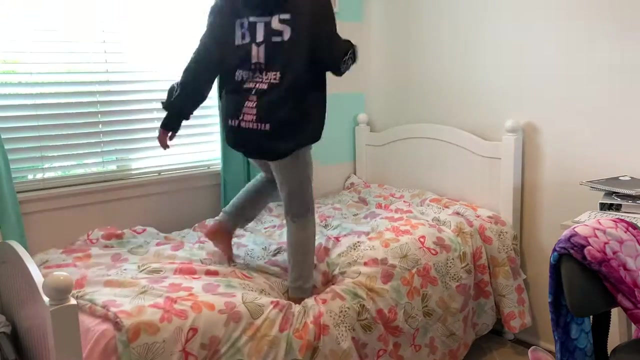 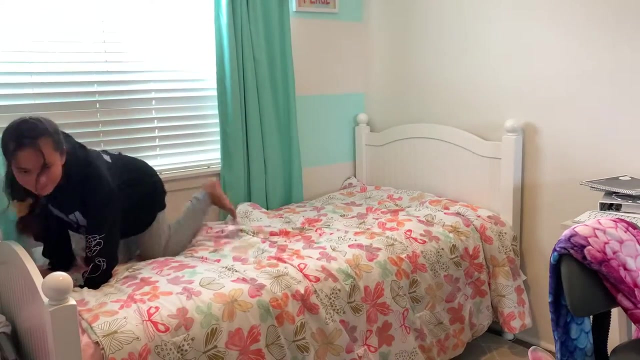 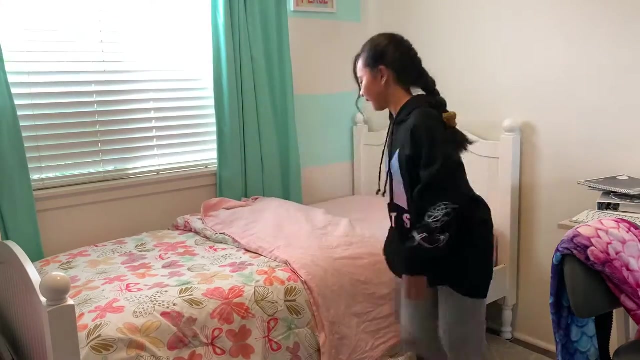 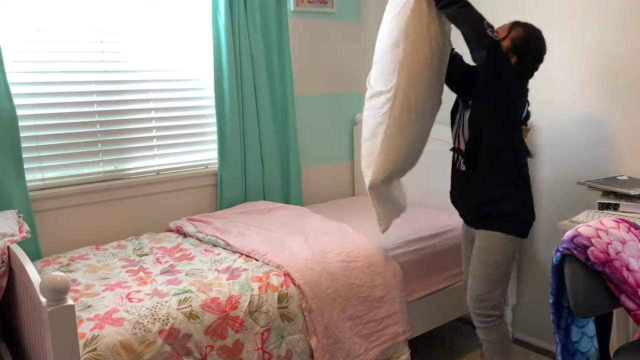 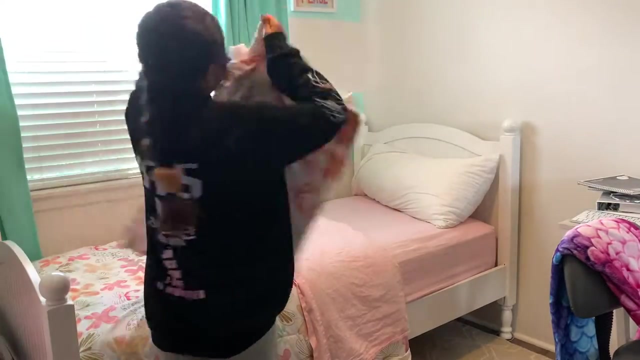 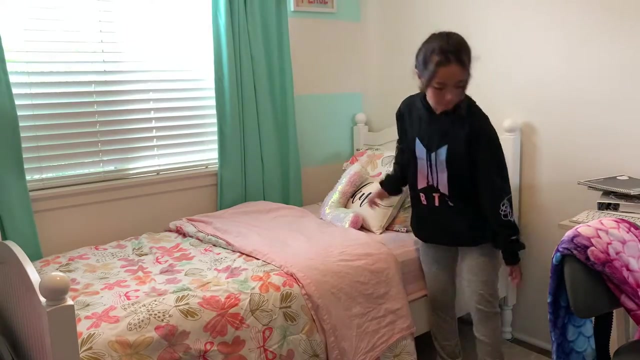 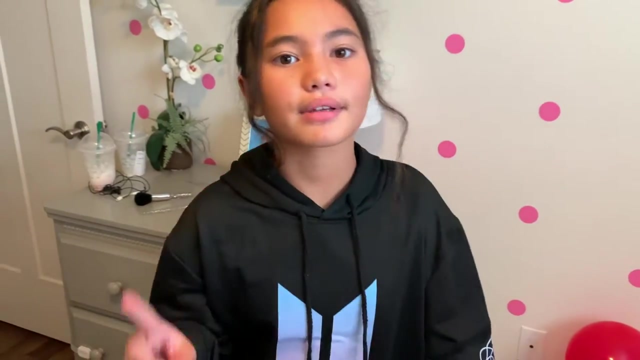 it's time. one, two, three. okay. so one, two, three, four, three, four, five. Why do I have so much bedding? and we're making this look easy cuz it's not 2,000 years. Okay, guys, so now for the next step. we're gonna do my sister's bed. 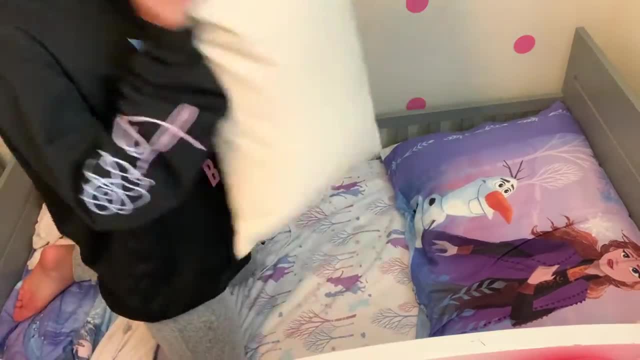 Okay, guys, I'm confused. Why do I have so much bedding- and we're making this look easy, cuz it's not 2,000 years. There's so much stuff in her bed- I Mean she's only three and she doesn't even sleep in it. 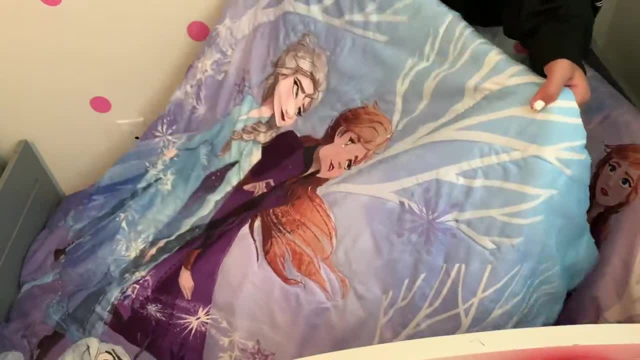 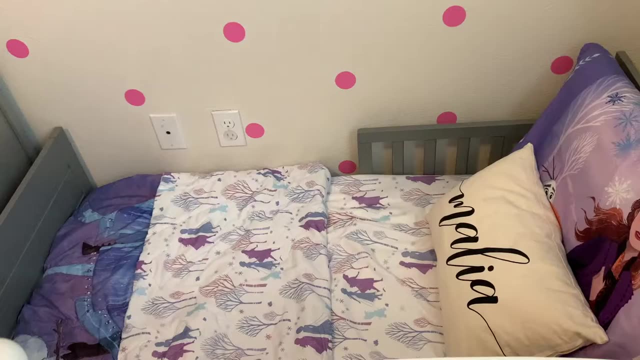 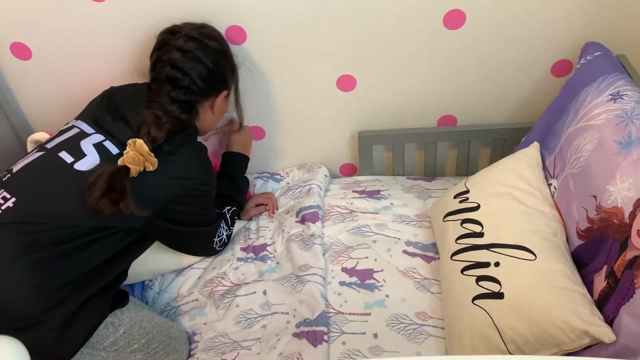 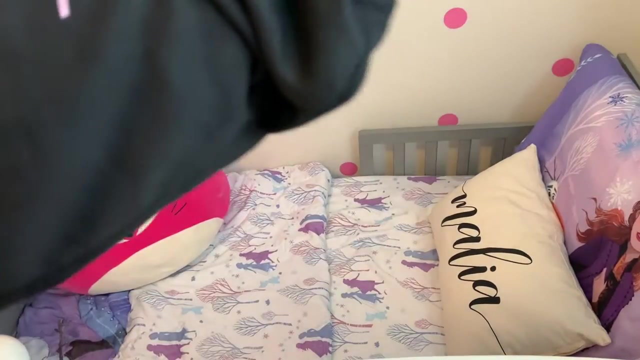 As you can see, it's really tricky to fix her bed because It's really tiny and there's not a lot of space for me to work with this, And the best sister award goes to me for putting the outlet cover on the outlet safety first. Another pretend coffee break. 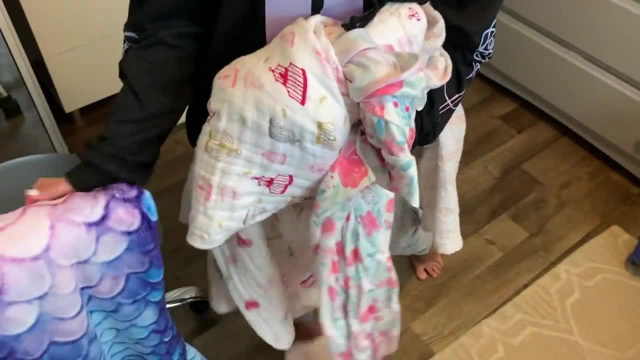 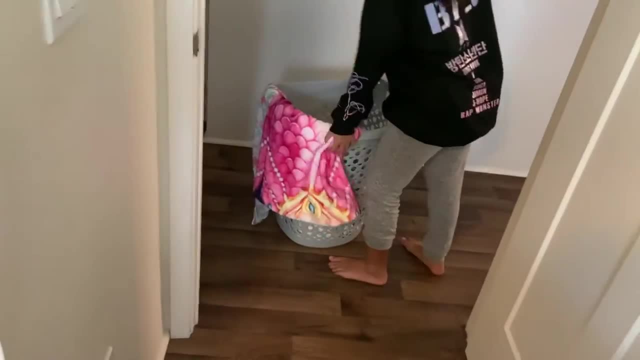 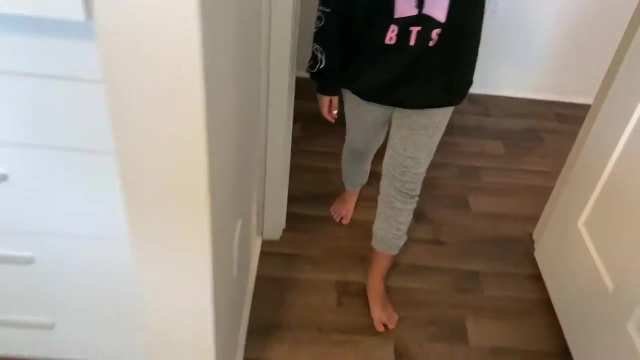 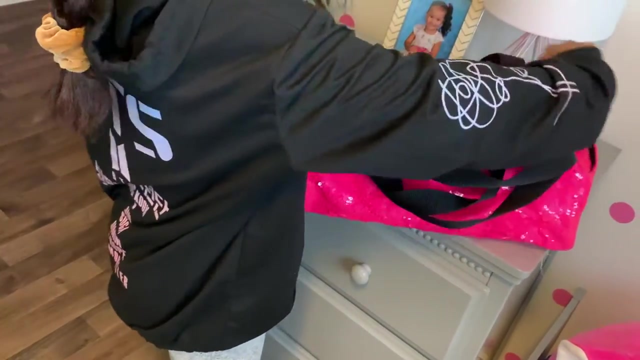 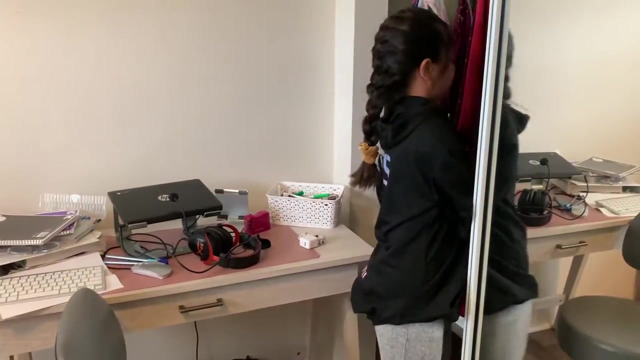 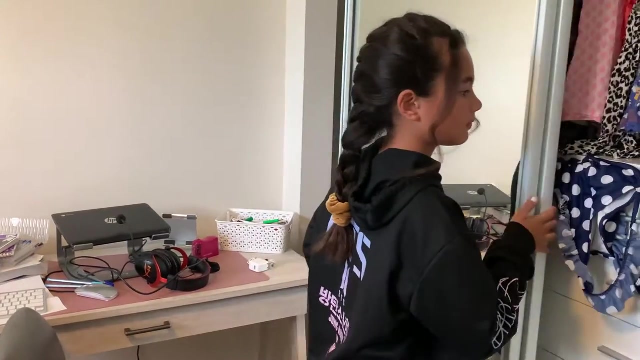 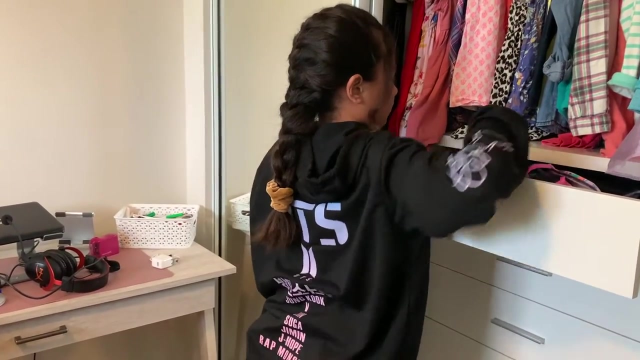 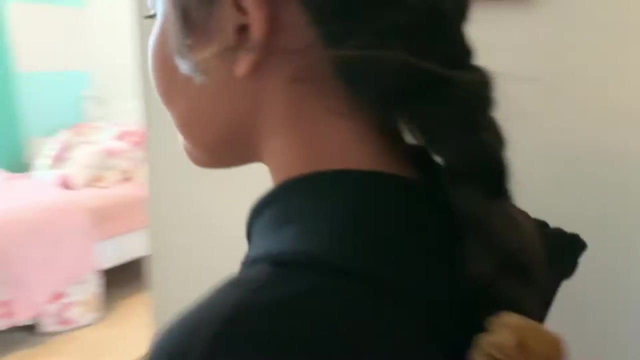 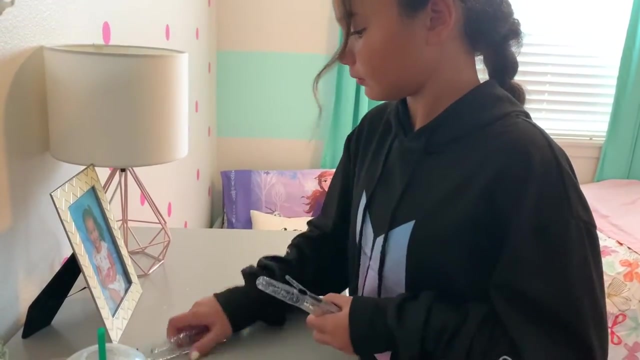 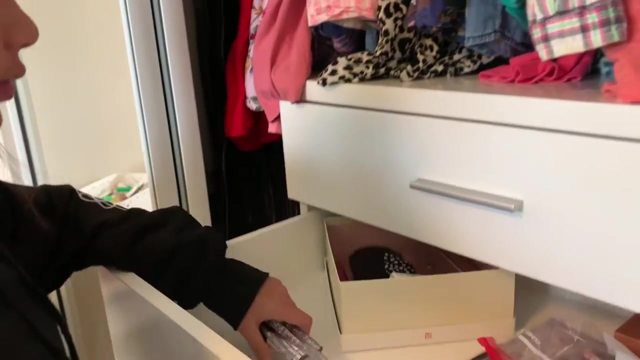 Now I'm just gathering all the blankets and putting them in the laundry basket. This is my secret bag where I hide all my favorite toys. Oh, I love my toys. In the closet it goes- Another pretend coffee break. Don't mind me trying to organize all these boxes. 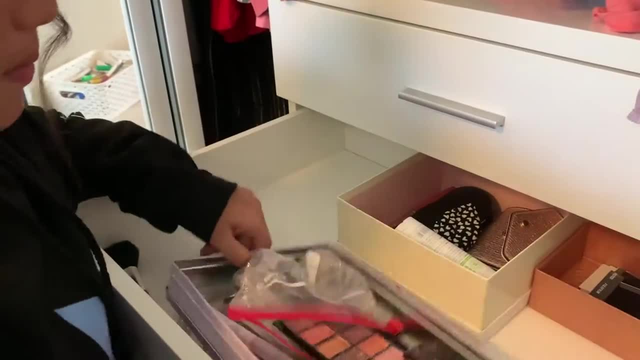 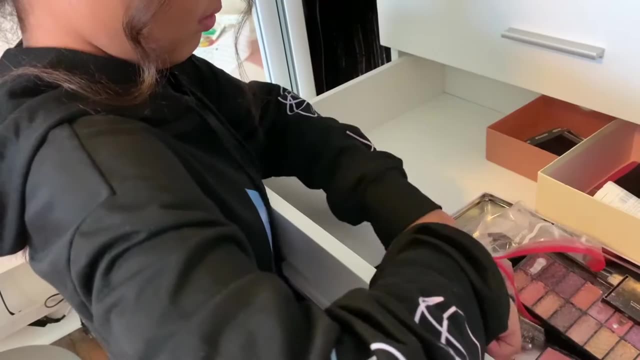 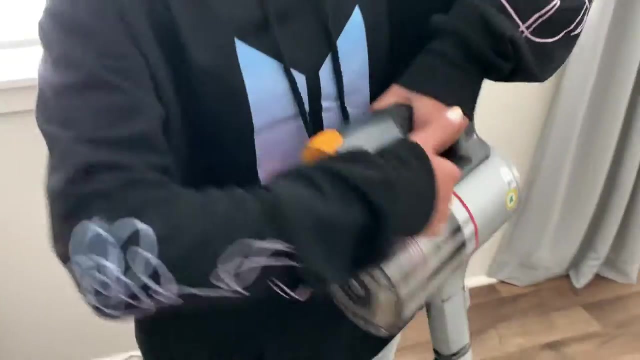 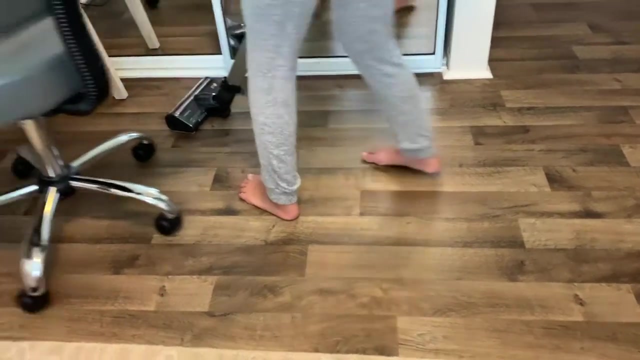 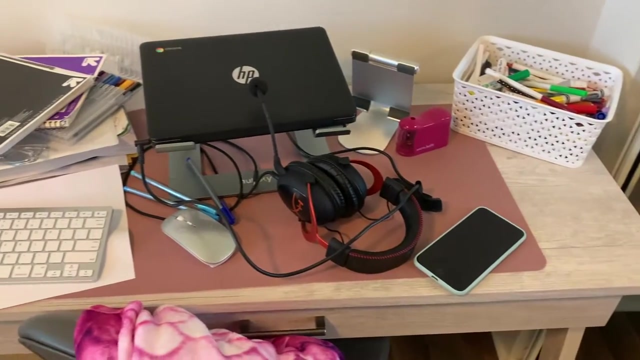 It's kind of like a puzzle. I'm just going to vacuum up all the pencil shavings and put them in the closet. I'm just going to vacuum up all the pencil shavings and put them under my desk. Yikes, I don't know whose desk this is. 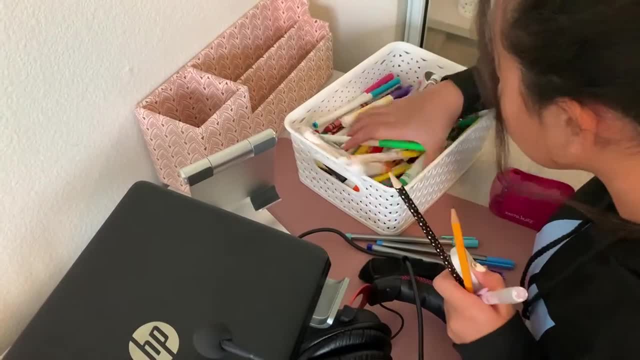 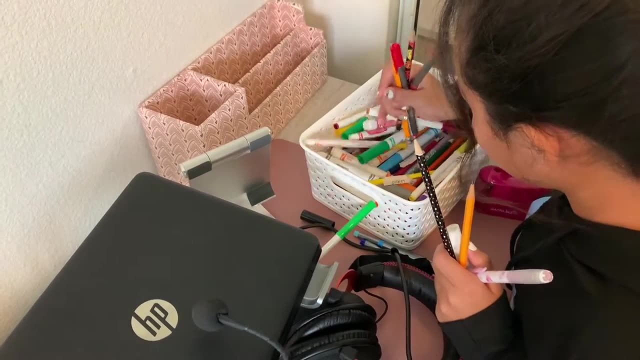 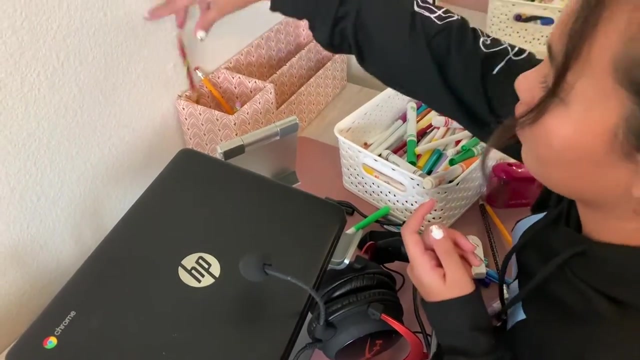 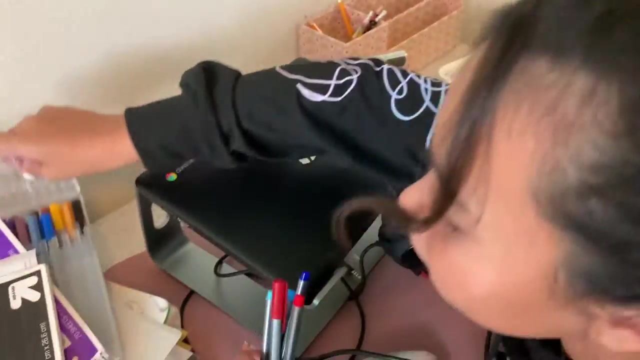 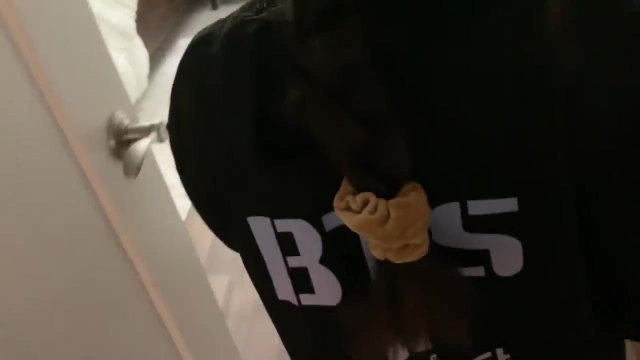 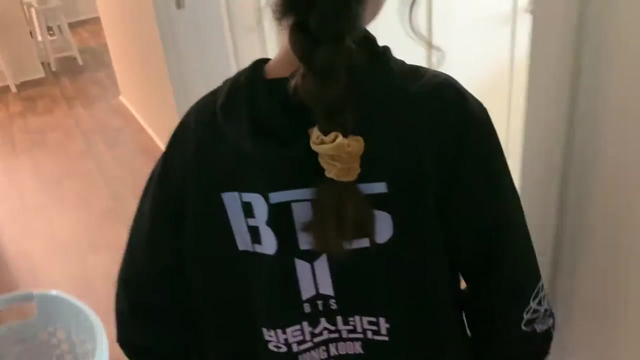 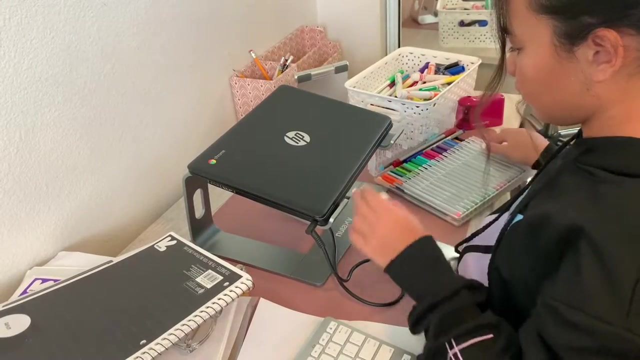 but it's not mine. Let's start with organizing all my pencils first. Let's start with organizing all my pencils first, And let me put my headphones away so I have more space to look. Now let's just clear everything out of the way. 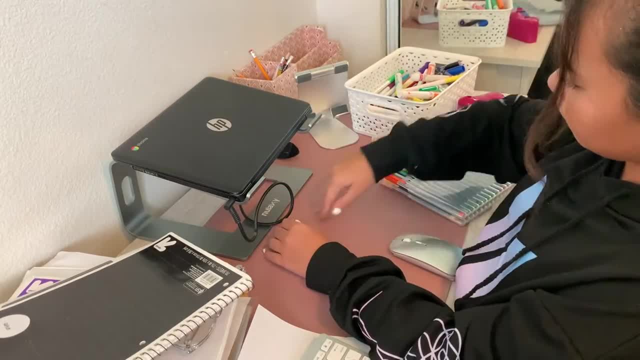 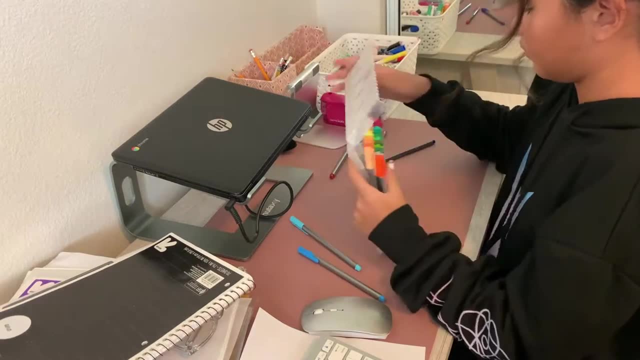 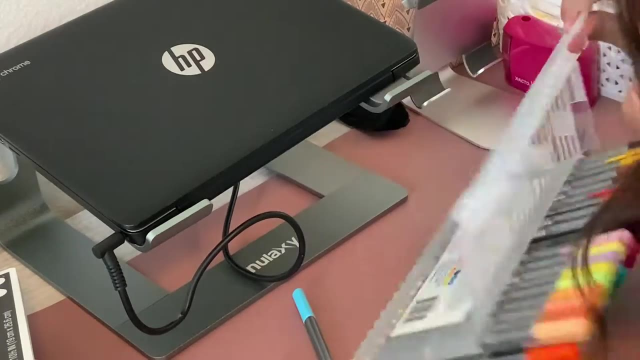 Now let's just clear everything out of the way. Now, let's just clear everything out of the way. This is a 40-pack of pens from Target. I love that it came with its own pen case. It makes it super easy to organize. 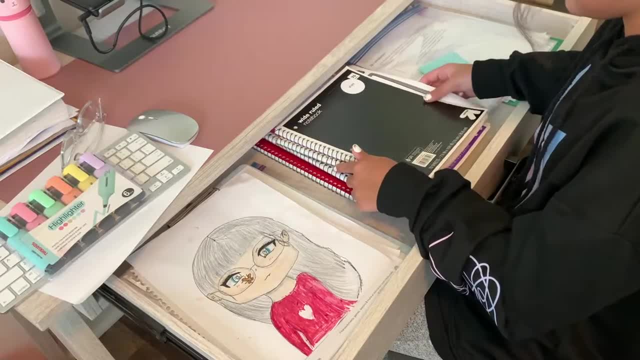 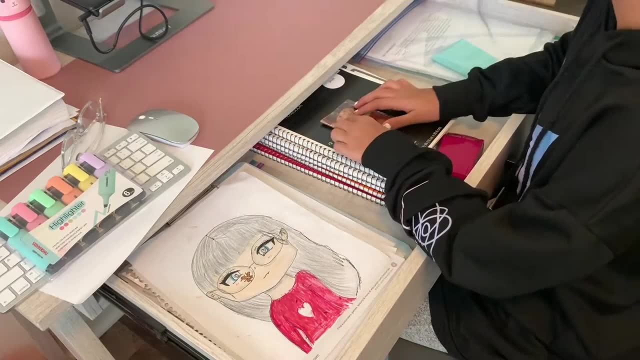 Now I'm just putting everything inside the drawer, So that drawing that you see here it was a recreation of a friend's drawing You can see over there. it was a recreation of my friend's drawing- A little picture of me and my mom and dad. 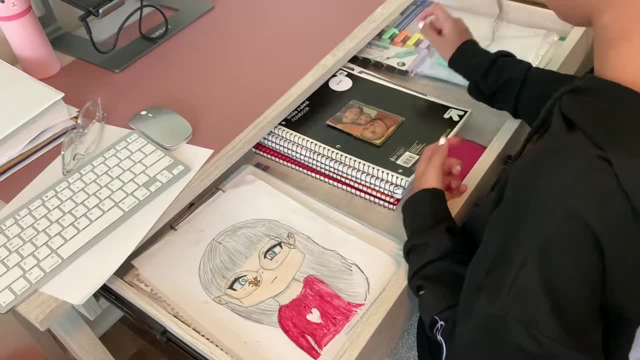 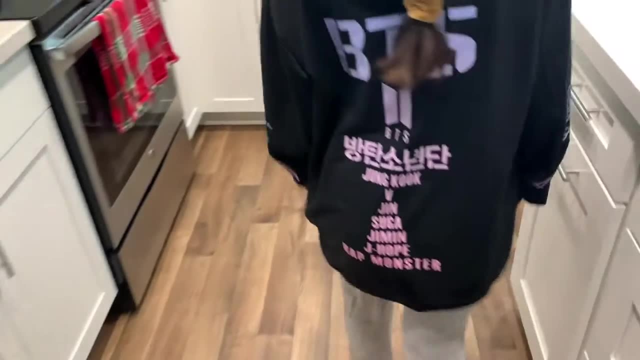 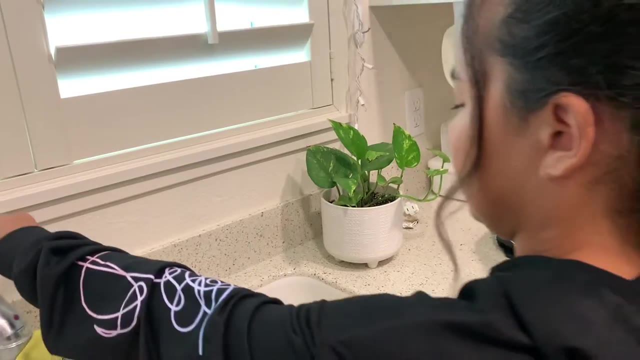 from when I was little, And my pastel highlighters And, of course, my blue light glasses. Now I'm just grabbing a rag. Now I'm just grabbing a rag to wipe all of the dust off of my desk. to wipe all of the dust off of my desk. 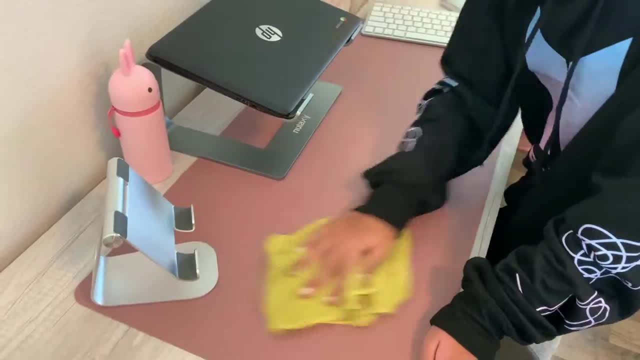 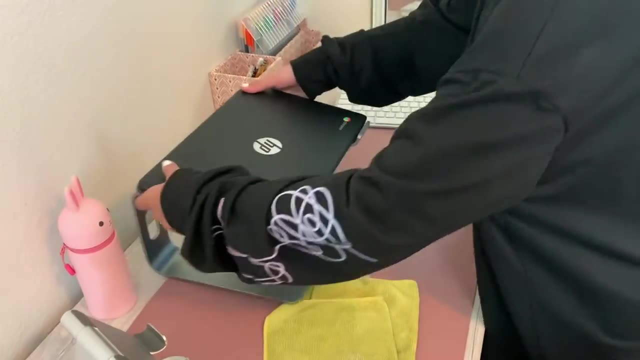 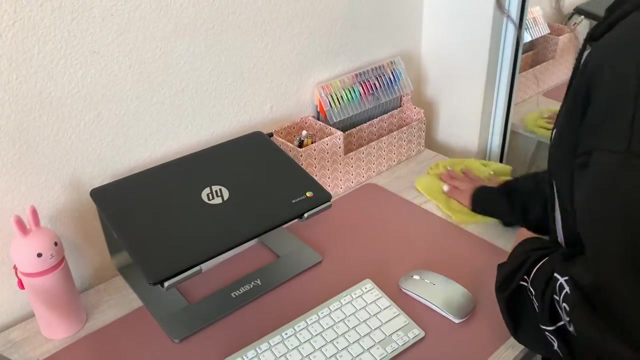 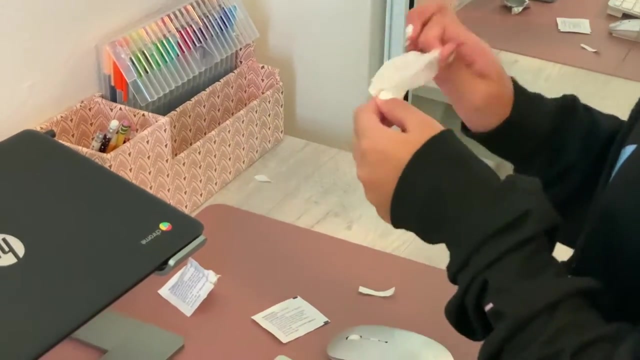 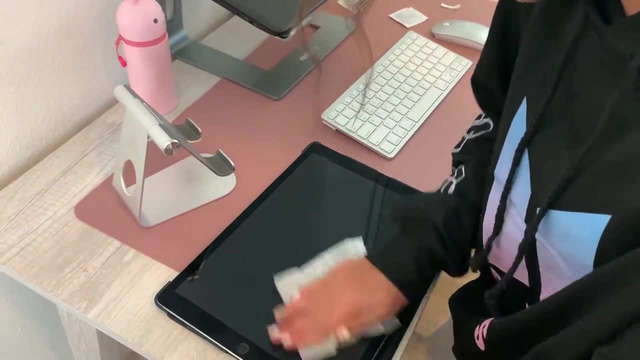 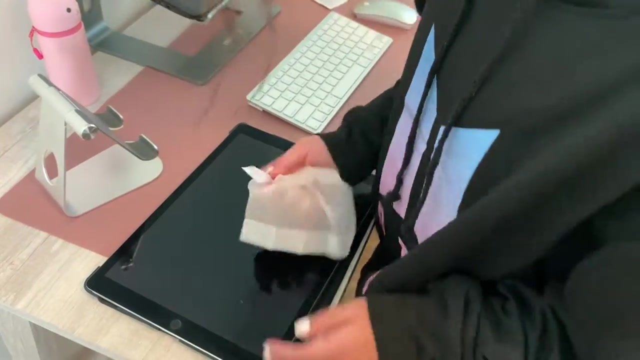 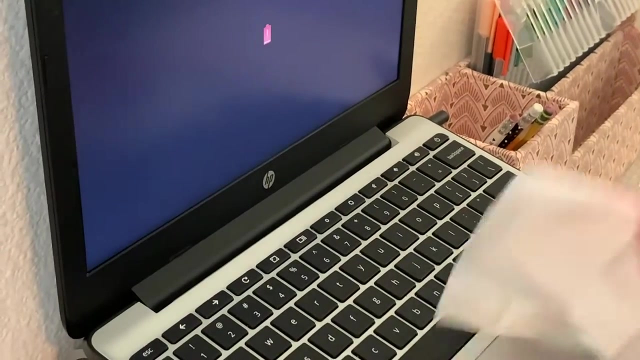 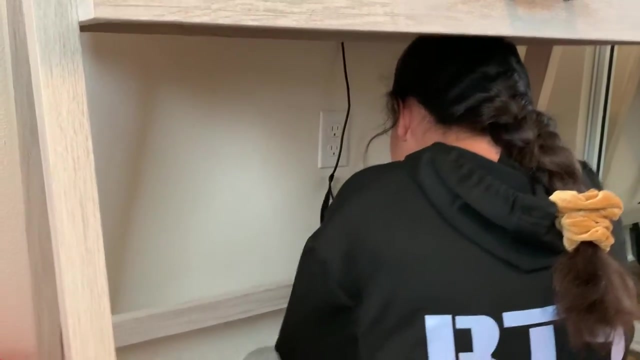 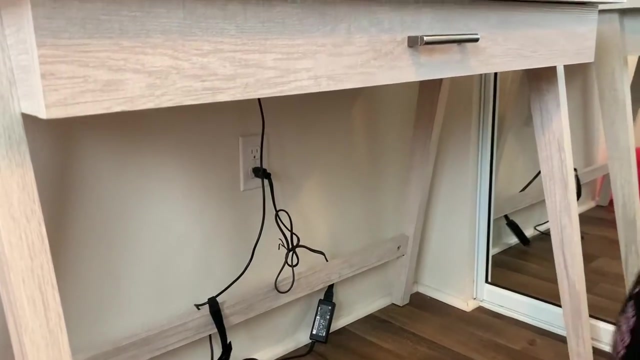 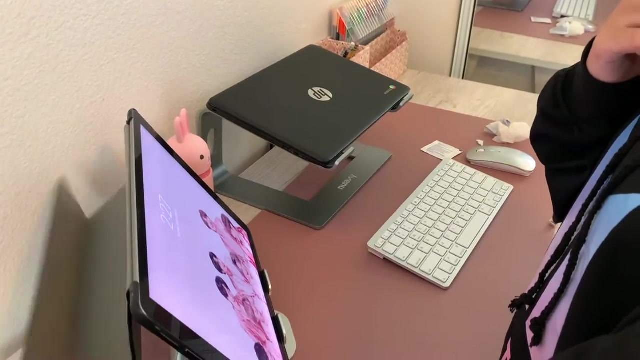 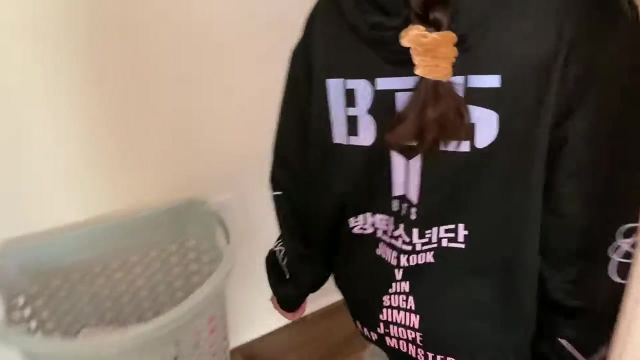 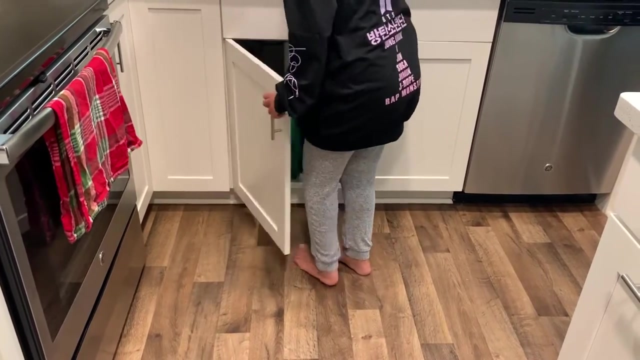 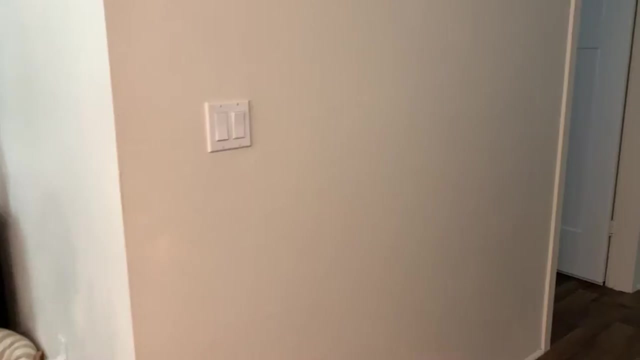 And I'm just using a special wipe to wipe all of the fingerprints off of my iPad. Oh, my Chromebook is dead. I'm just going to go plug it in. Now. it's time for me to clean my mirrors. I'm just grabbing the window cleaner and a rag. 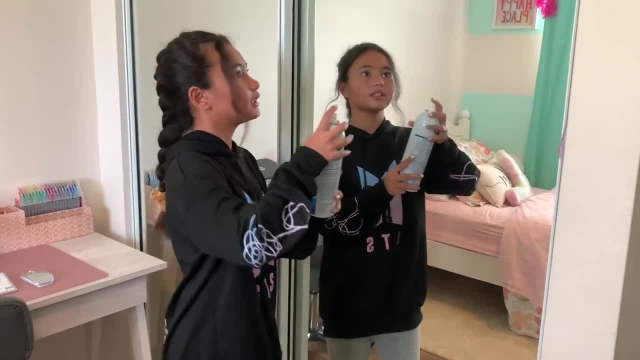 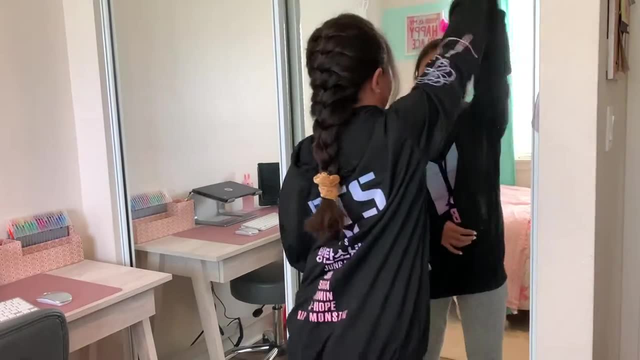 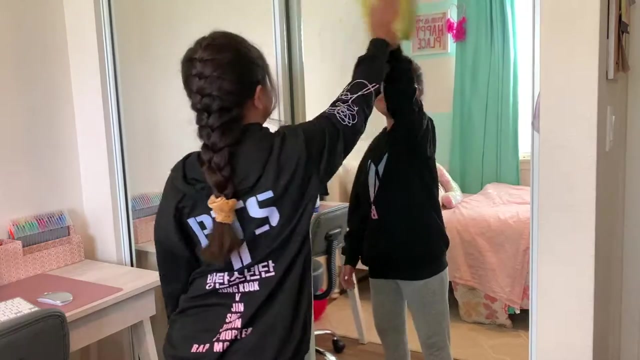 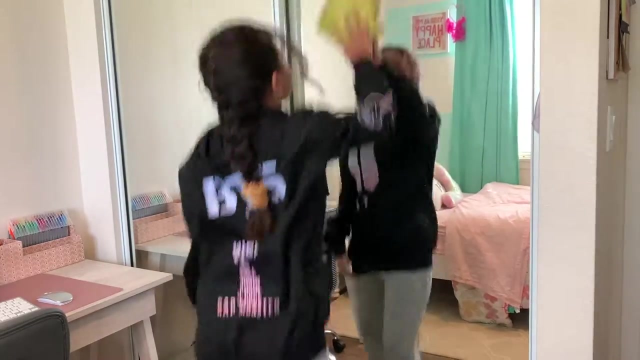 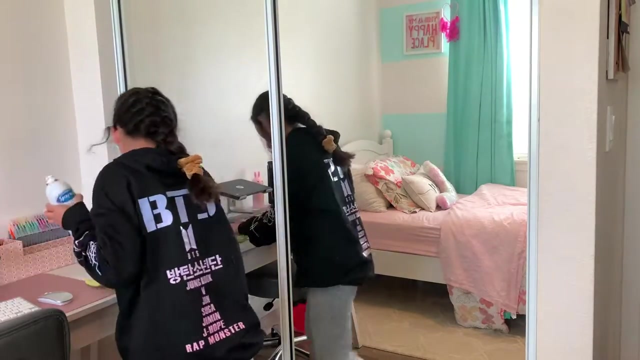 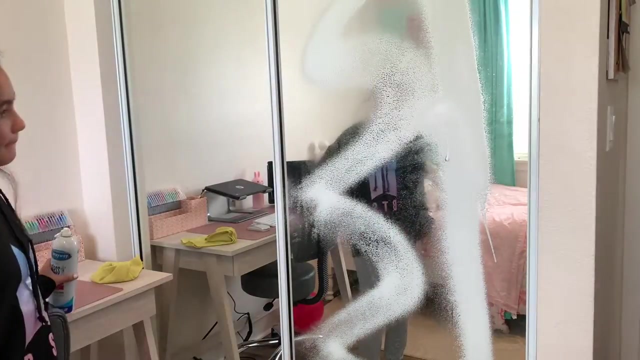 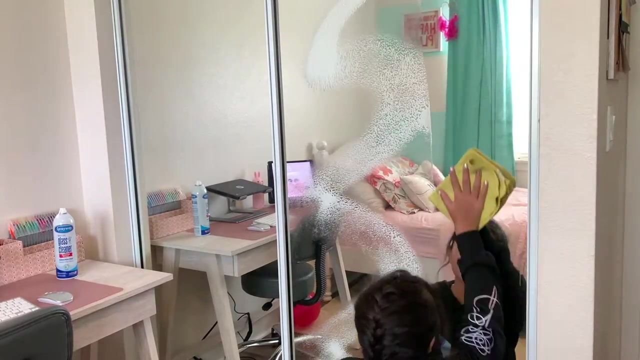 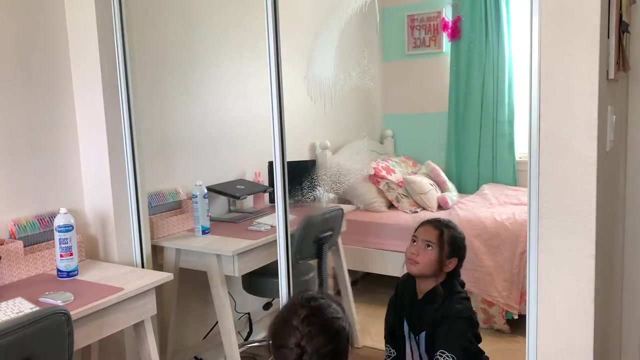 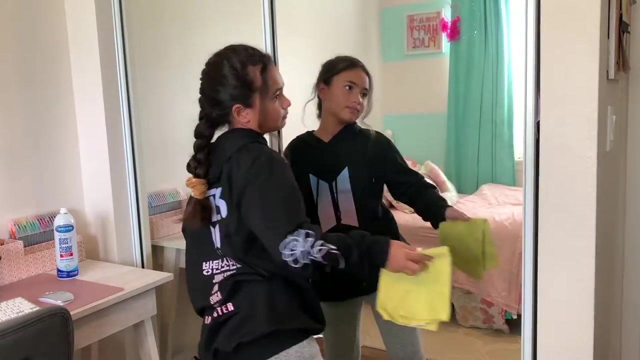 Oh my God, And I just held it there. Oh my gosh, it's so cute. I agree, man. It's so cute. That's so cute. All right, everything looks good. I'm going to put this away and throw away my trash. 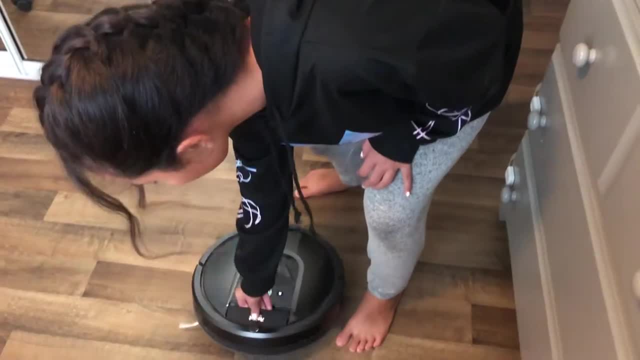 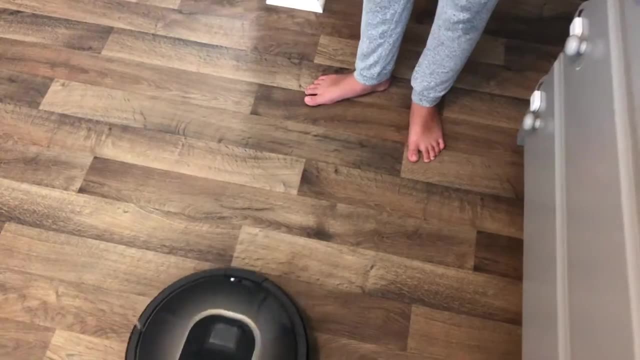 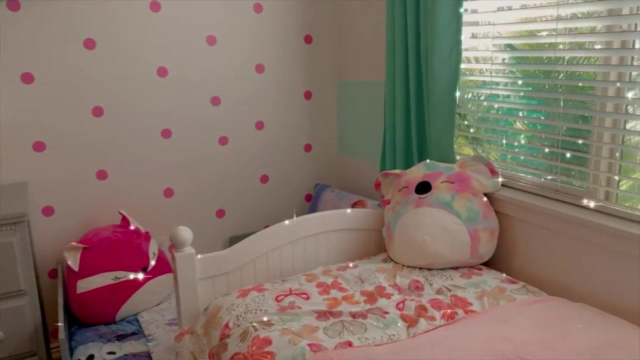 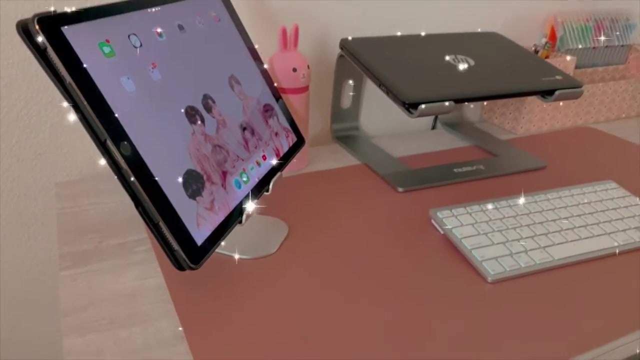 I know I vacuumed earlier, but I didn't vacuum everything, So I'm going to use a Roomba to vacuum all of it. All right, I'm all done. My room is sparkling clean. This is my desk area. All right, guys, that's it for this video.